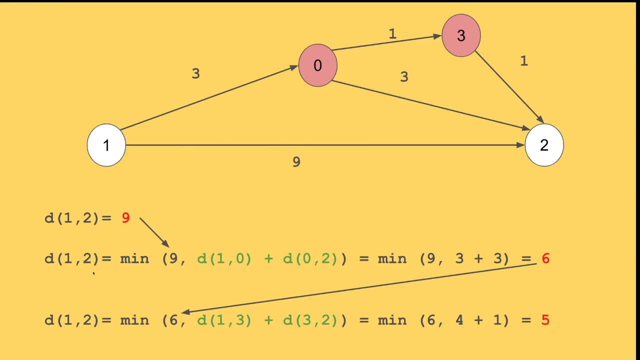 this one, I can say. the distance can now be updated to the previous distance, which is 6 plus the shortest distance of going from 1 to 3 and then the shortest distance of going from 3 to 1.. This value would be 4 plus 1. 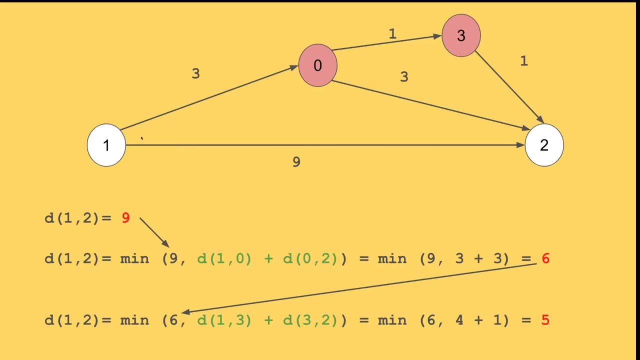 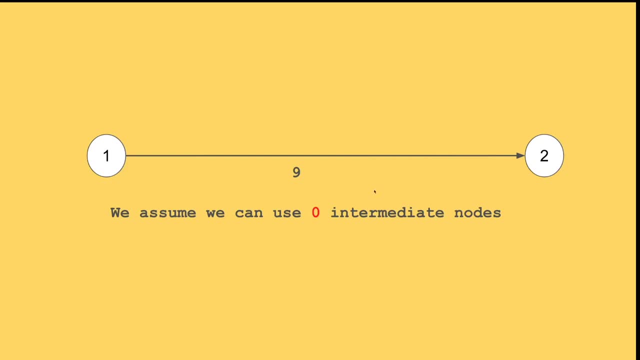 and then the minimum of 6 and 5 would be 5,. therefore I can go from 1 to 0, then to 3, then to 2 at a cost of 5.. So you see that I sort of give you no node, no. 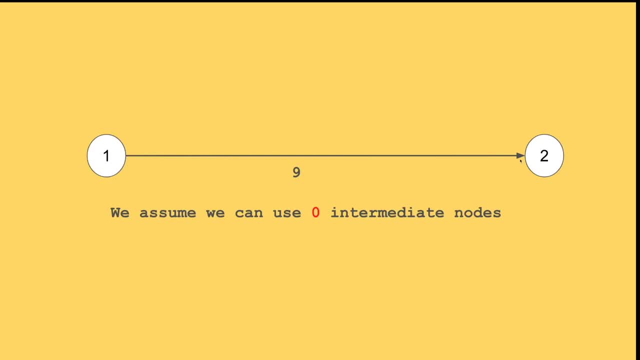 intermediate node in the beginning so you can say I can go directly. then I tell you: hey, you're allowed to use only one node between 1 and 2, so you can update your distance to 6,. then I gave you two nodes and then you could say, hey, I can update this value to 5.. In the extreme I can. 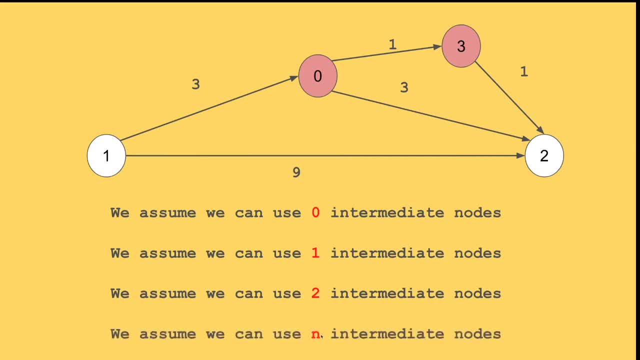 give you. you're allowed to use all n nodes as an intermediate node. therefore, you have much more freedom. therefore, if we repeat this from 0 to 1 to 2 and then to n, the shortest path at the end should be the actual shortest path between 1. 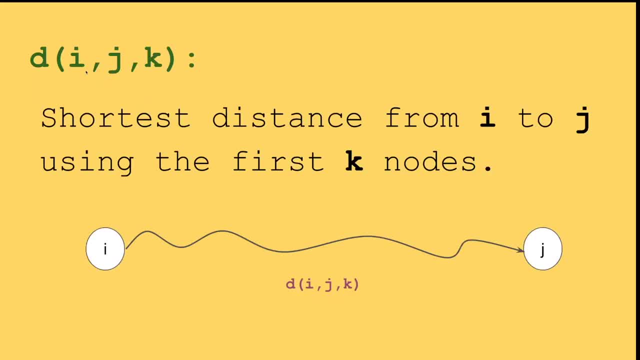 and 2.. I can generalize this and say the shortest distance between all i and j using the k first nodes is shown by d of i and j and k, a function with three parameters that shows the shortest distance of going from i to j using the. 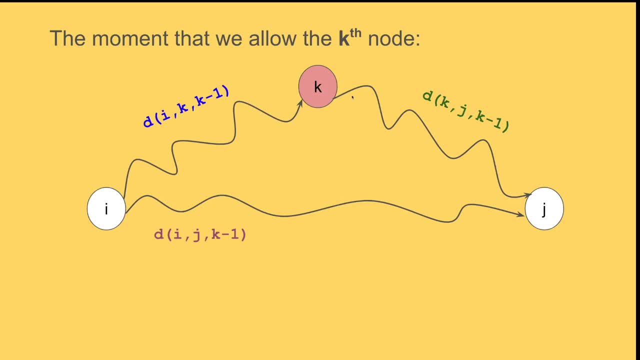 first k nodes And then I can generalize the moment that I'm adding the kth node. and I can say, whenever you're adding the kth node, if you are comparing the case of going i to j with only k-1 nodes to the case that I go from i to k first using k-1 nodes and then 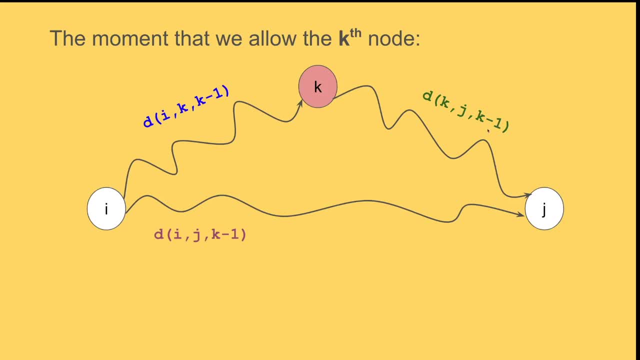 I go from k to j using k-1 nodes And then I can generalize this minimum value that we calculated, which takes the minimum of this path, the direct path between i and j using k-1, and then i to k plus k to j, And I can sort of come with this. 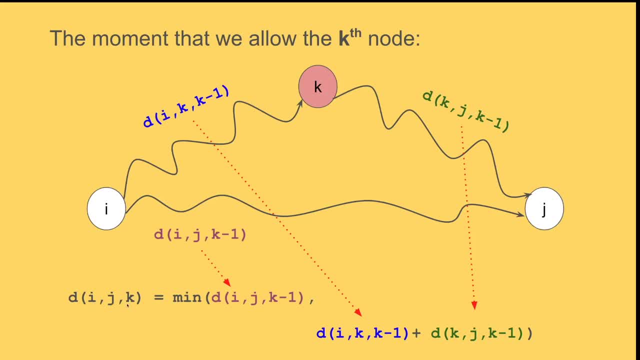 recursive value. If you notice, the d of i and j and k now depends on d of i- j- k-1,, d of ik- k-1, and d of k- j- k-1.. So each time k depends on a value of k-1. 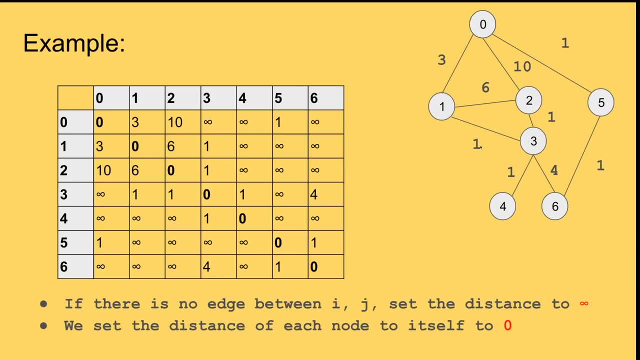 Alright, so now let's see an example. So this is a graph, it's a bigger graph and the first thing I do is to create a matrix that shows the edge values, the weights between each i and j, For example, between 0 to 1, the edge value, the weight, is 3.. So 0 to 1, I. 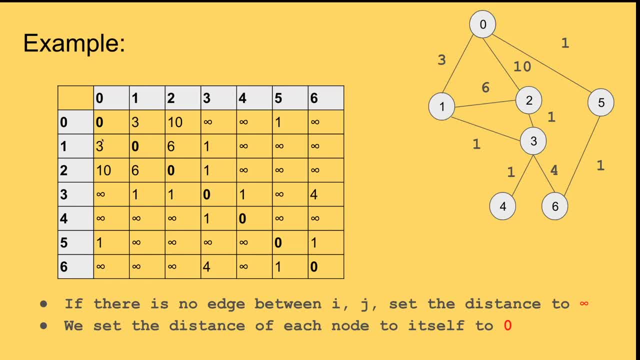 put 3.. And I do this for all the edges, and I put 0 to represent the shortest distance between each node to itself. So 1 to 1,, 2 to 2, everything on the diagonal would be 0. And then, if there's no edge between two nodes, for example between 0 and 3, there's 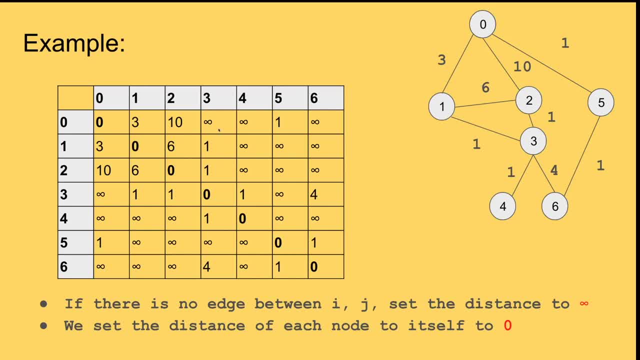 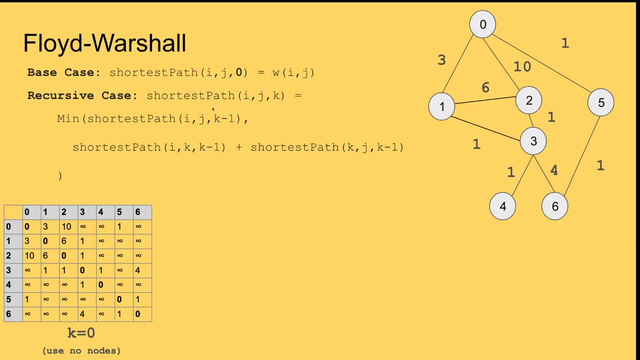 no edge. I can put an integer, I can put an infinity to represent that. So this matrix, this initial matrix, is a direct translation of our graph. We haven't calculated anything yet, And let's write our recursive function that we just came up with here, And I'm showing you, on the bottom left, the case. 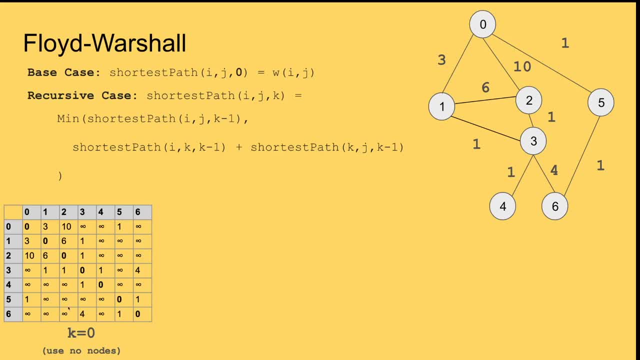 where you're not allowed to use any intermediate node, where we start from Now in this graph. if I tell you now you are allowed to use node 0 as intermediate, there are certain i and j, certain nodes that 0 is between the path between i and j is on the path between. 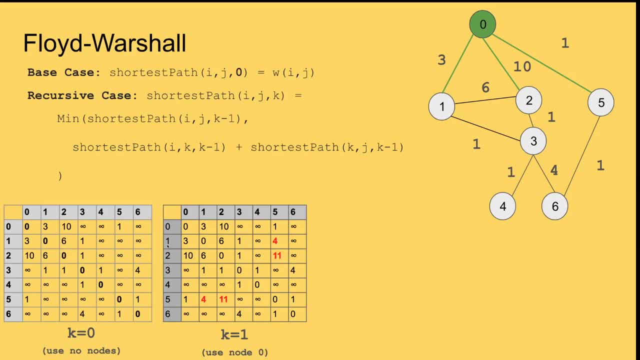 i and j, which we can update, For example, between 1 and 5, there's no edge. So the path, the shortest path of 1 and 5 was infinity. Now using, when we are allowed to use 0,, the. 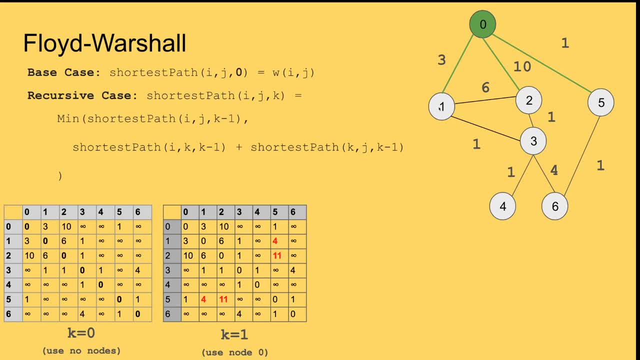 shortest path between 1 and 5 is going from 1 to 0, 3, going from 0 to 5, 1.. So the value gets updated To 4.. There's one more update that we can do, which is node 2 to 5.. 2 to 5 used to be infinity. 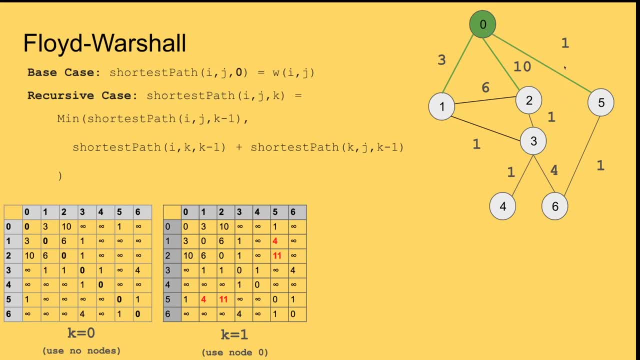 now I can go from 2 to 0, then 0 to 5, and that would be 11.. And remember: so far we are only allowed to use node 0 as intermediate value. Now I repeat this one more time. So with this new node 1, I'm not allowed to use node 0 and 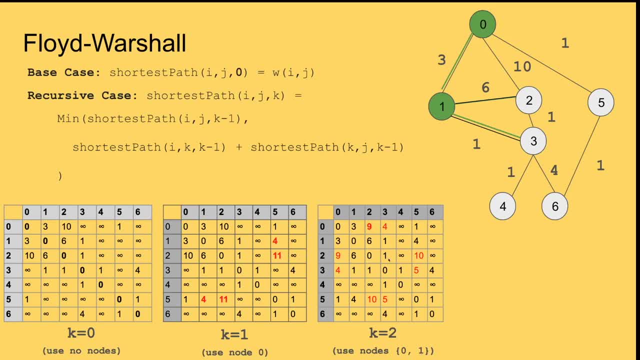 1 intermediate values, And this way I can go through all i and j and see what are the values that I can update, For example, for 0 to 2, I used to go from 0 to 2 by 10, but now I can go. 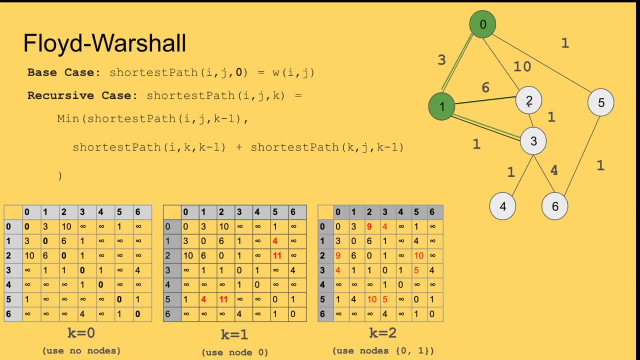 through 1, so 0 to 1, and then 1 to 2.. That would be 9 rather than 10.. Let's look at one more case, which was 2 to 5.. It used to be 11.. Now I can go from 2 to 1, then go to 0, then go to 5 for a. 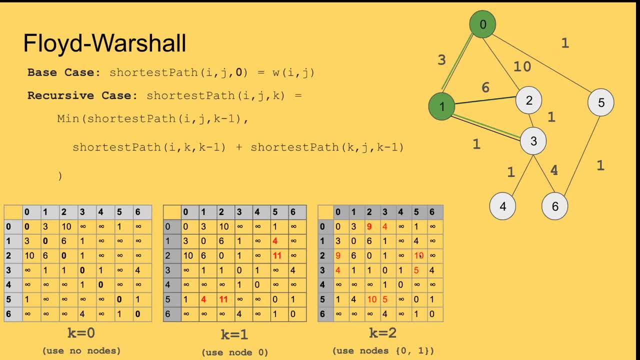 cost of 6 plus 3 plus 1,, which is 10.. So I can keep doing this and then use the new nodes each time And then, once I use all the nodes, this matrix will get the shortest path between all i. 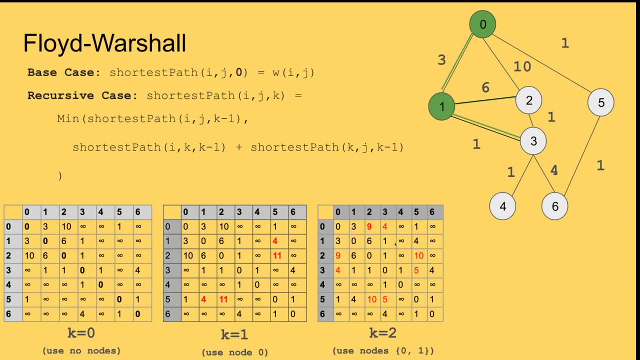 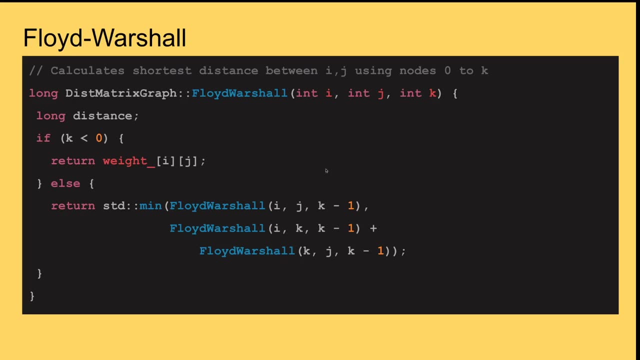 and j, And this is that is it. That is the insight of Floyd Warshaw. There's no other magic or tricks. All we do is to add intermediate nodes one by one and update this matrix. This is a translation of that formula in C++. You can write it in: 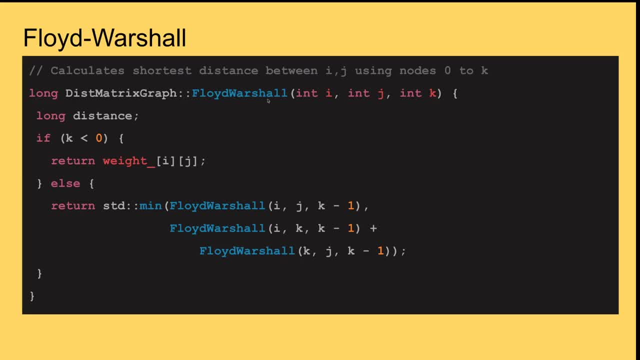 any other language. So I'm writing a recursive function which calculates the value of i and j and k based on i, j, k minus 1,, going from i to k with k minus 1, and then going from k to j with. 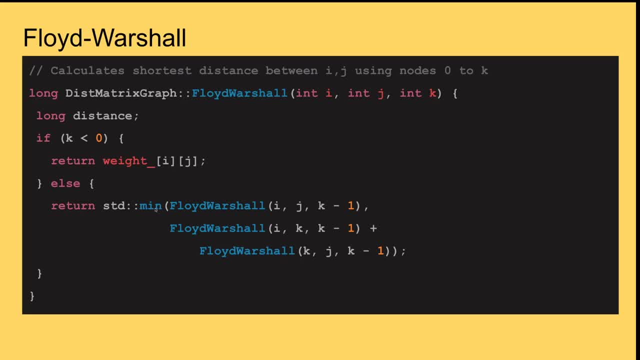 k minus 1.. So I'm going from i to j with k minus 1, and then going from i to j with k minus 1.. We add this together and then we calculate the minimum, And this is representing k represents: 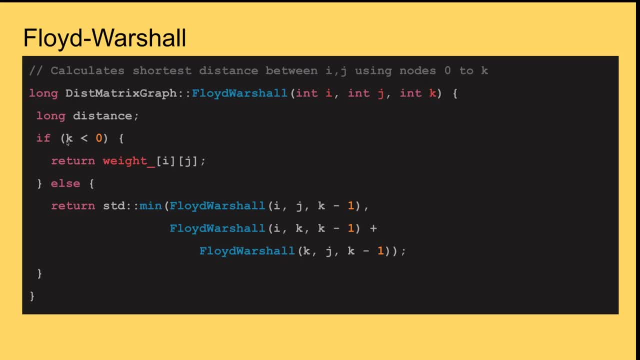 using nodes 0 to k. Therefore, our base case would be when the k k is less than 0, which represents you're not allowed to use any intermediate nodes. Therefore, the value should be the direct edge between i and j, And that's it. That's all what Floyd Warshaw is Now. this is a recursive. 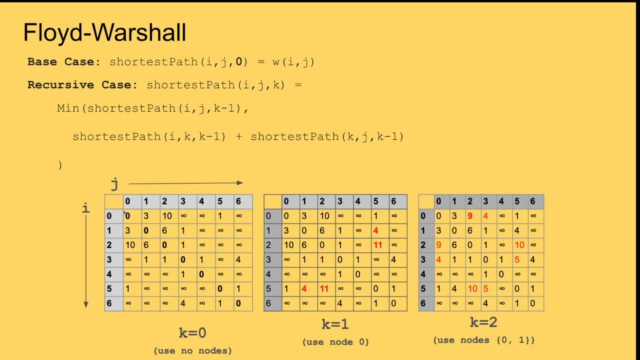 function. You can take the recursive function and say: well, I was iterating through i and j for updating this matrix each time, So this iteration looks like we are having two loops, one for i, one for j, And then I was doing updates on. k is equal to 0,. 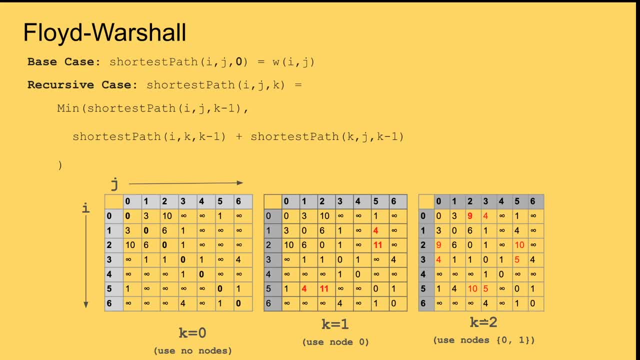 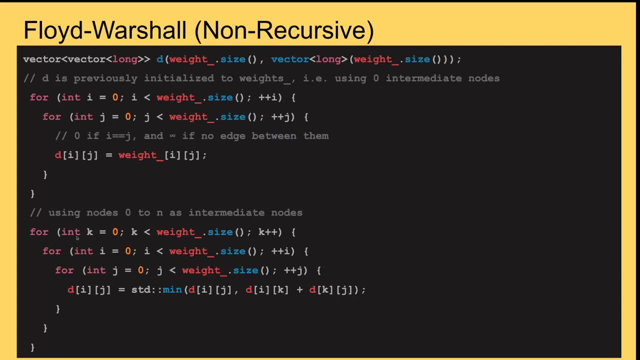 k equal to 1, k equal to 2.. That represents another for loop. So maybe we can come up with three for loops, one inside the other. The first one is iterating through k. Second one is iterating through i. Third one is iterating through j, And then each time, 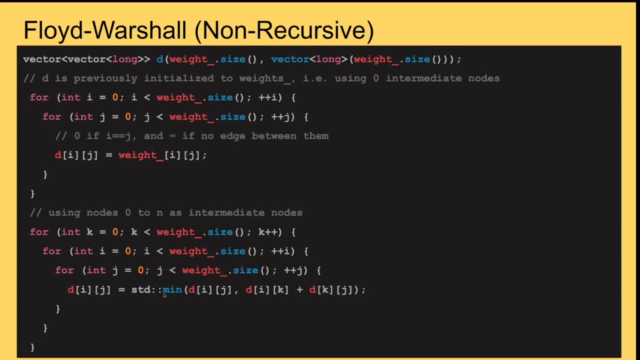 I can say the new matrix value of i and j is equal to the minimum of the previous value, the previous shortest path between i and j comma, the shortest path, the previous shortest path of going i to k plus going to k from k to j. So that's the main, that's the meat of the 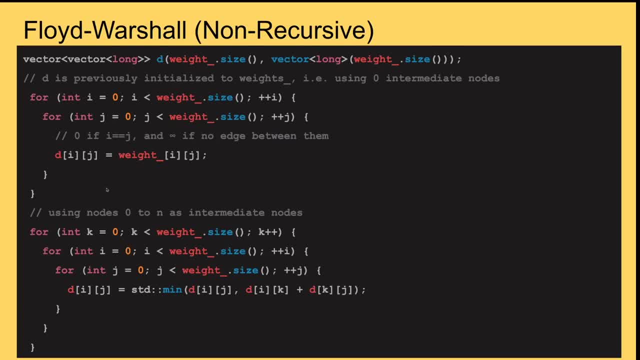 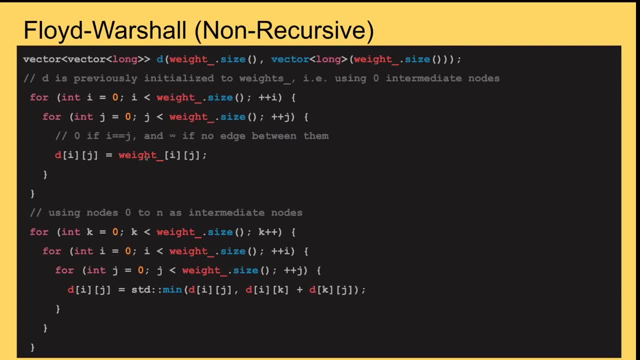 i is equal to 0.. I'm not exactly showing this, but these weights are initialized. If i is equal to j, the i, j is initialized to 0. And if there's no edge between them, they initialize it to infinity or a very large value. in your program It can be a very large integer. 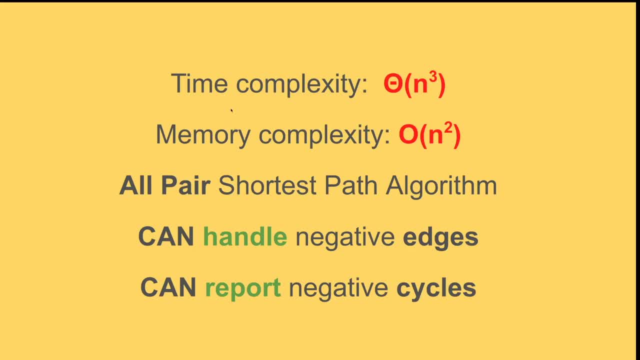 A summary of what properties this algorithm have. So you saw, we already have three, four loops. Therefore the runtime complexity is theta of n3.. Memory complexity: we have n by n matrix. Therefore it's all n2.. We are calculating all pair. It's the shortest path. 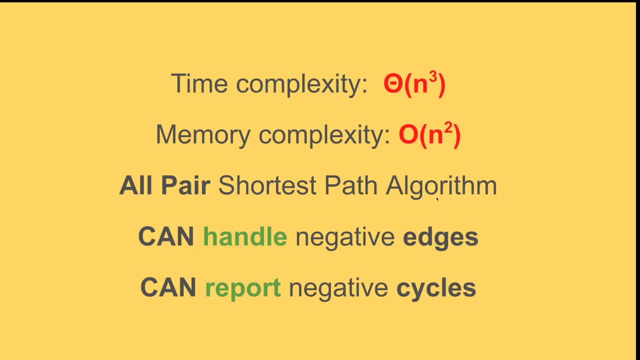 between each i and j, So it's called all pair shortest path algorithm. We didn't talk about this, but just be aware that it's okay in this algorithm to have negative edges. This algorithm still works, still handles it, as long as you don't have negative cycles. And remember, if you have 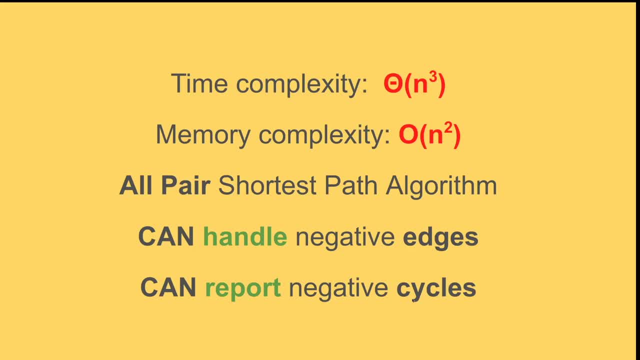 negative cycles, the shortest path cannot be defined. It doesn't mean it's not going to be defined. So it's going to be defined. So it's going to be defined. So it's meaningless to define a shortest path if there's a negative cycle reachable from your.